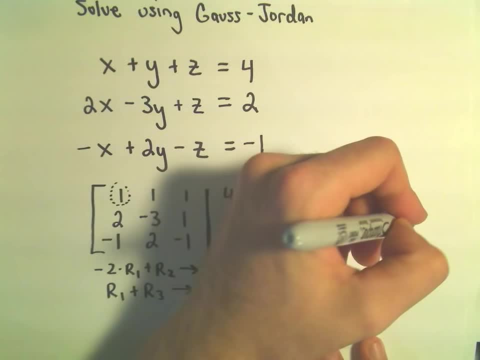 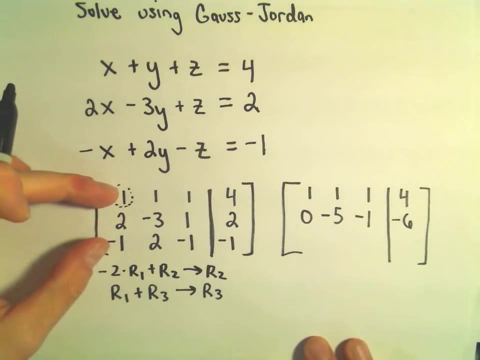 We'll get a negative 8 plus 2. Which will be negative 6.. And then, to do our last one, we just add row 1 and row 3. So 1 and negative 1 will be a 0. We'll get a 1 plus a 2, which will give us 3.. 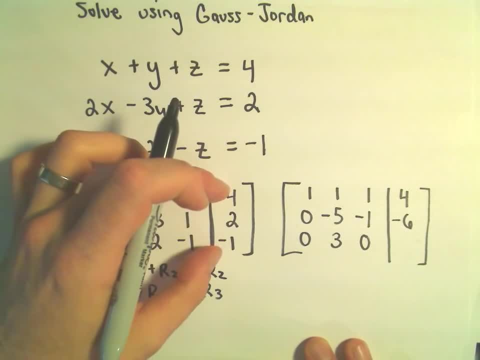 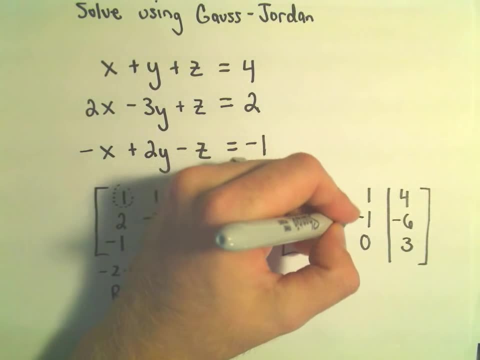 1 plus negative 1 will give us 0. And then 4 plus negative 1 will give us positive 3.. Alright, so the next thing I want to do is I want to make the middle entry into a 1.. To do that I'm going to, I think. 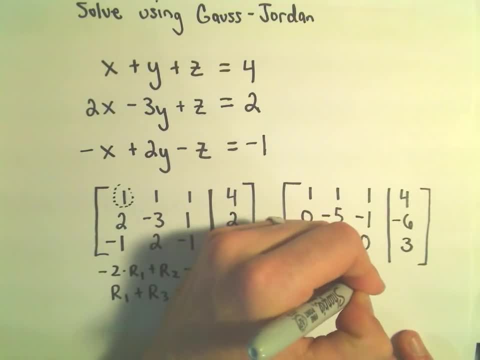 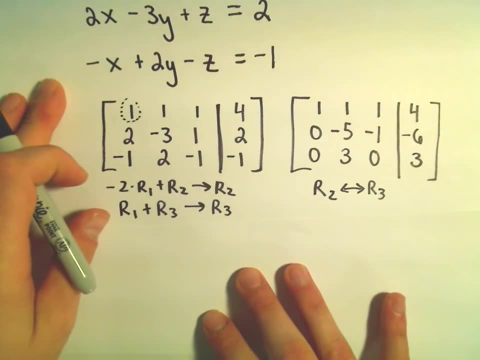 interchange row 2 and row 3.. I'm just going to switch those out. So if we switch those out, okay, it's not going to make the 1 appear immediately, but you know, we'll be able to just divide by 3 and then we'll get it. 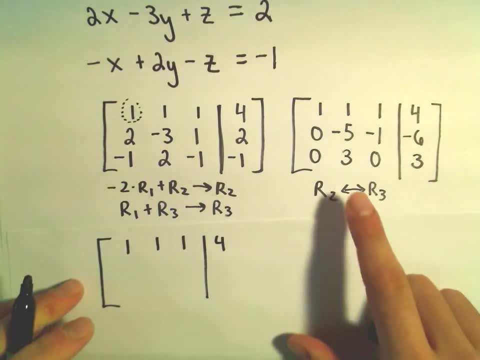 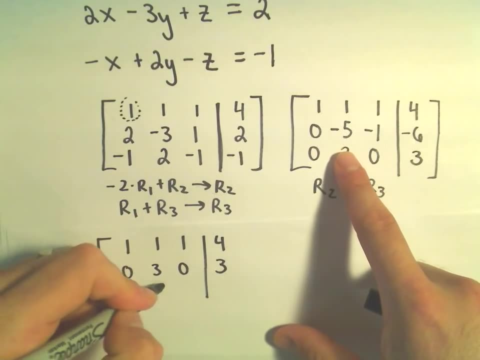 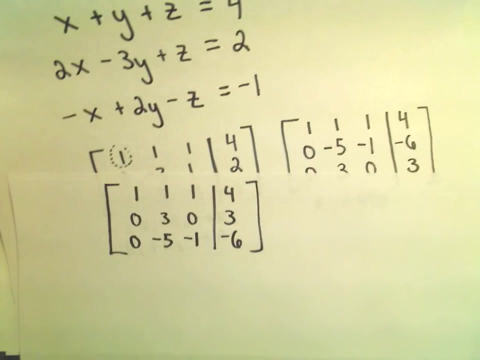 So we have 1,, 1, 1, and 4, leaving the first row alone. I'm going to write the third row now as my second row, And then the second row is going to become the third row. Okay, so again I'm trying to get. I want a 1 where this 3 is sitting. 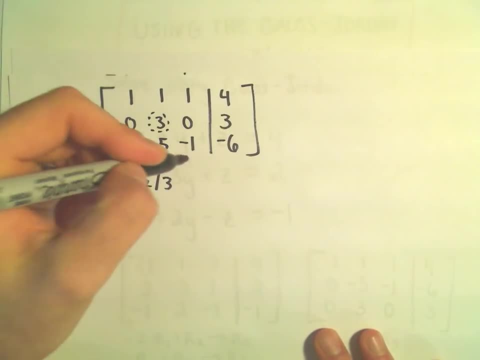 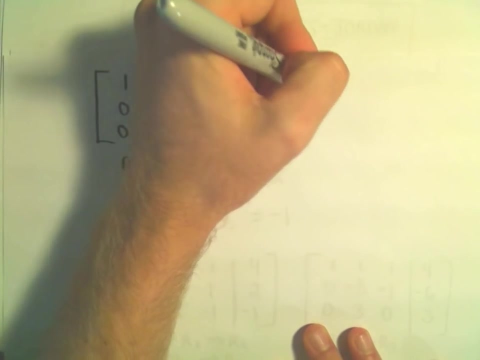 So I'm just going to take row 2 and divide that by 3, and that's going to become my new row 2.. So if we do that again, the first row is just hanging out: 1, 1, 1, 4.. 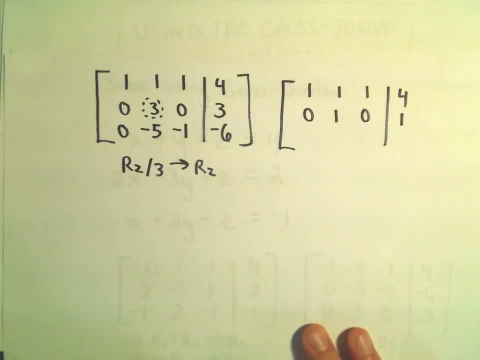 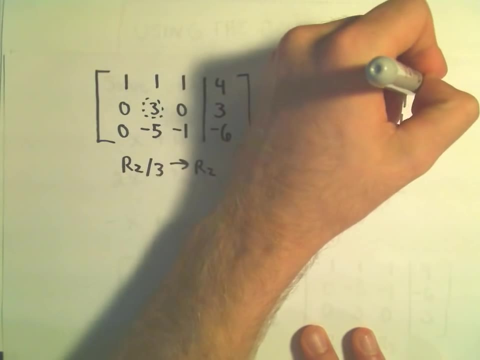 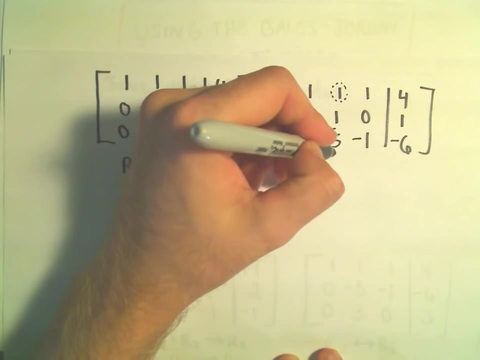 We'll get 0, 1,, 0, 1 for our second row. now The third row. we're still just leaving alone 0, negative 5, negative 1, and negative 6.. Okay, so now we want to get 0s in the first row and in the third row, in the second column. 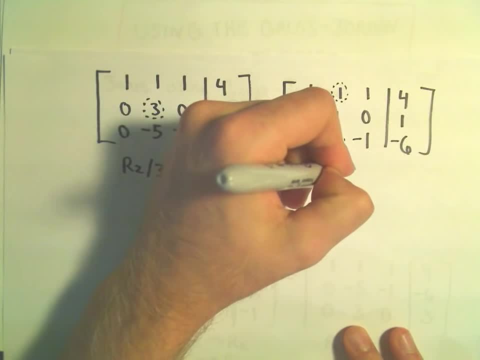 So what I'm going to do is I'm going to take negative 1 times row 2, add that to row 1 to get my new row 1, and then I'm going to take 5 times row 2, add that to row 3 to get my new row 3.. 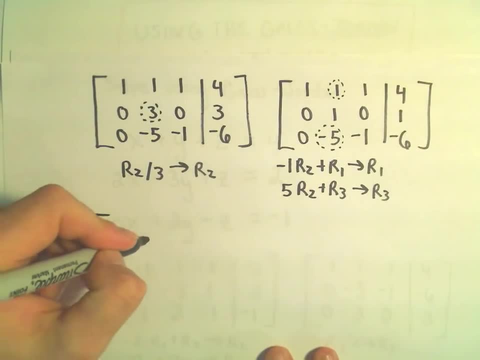 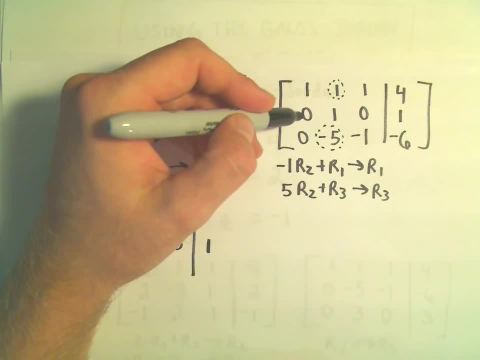 So let's see here, if we do that, So row 2, it's staying just like it was, so I'm going to go ahead and rewrite it. Let's see, we'll get negative 1 times 0 plus 1 will be 1.. 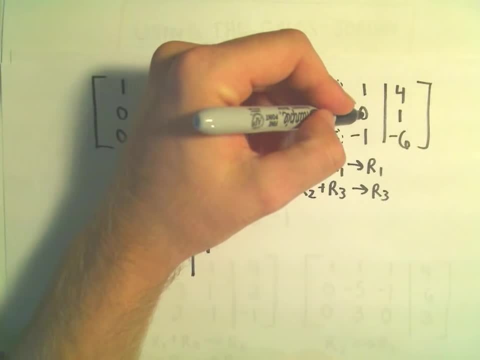 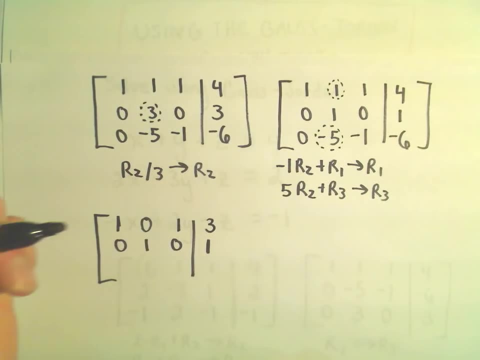 We'll get negative 1 plus 1,, which will be 0.. We'll get 0 plus 1, which is 1.. Negative 1 times 1 is negative 1, plus 4 will be positive 3.. And then let's see. so, if we do our second step here, 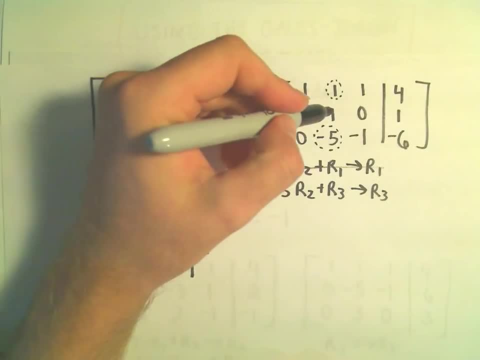 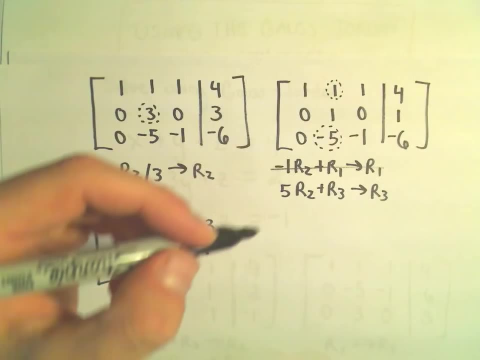 5 times 0 plus 0 is 0.. 5 times 1 is 5, plus negative 5 will give us a 0.. 5 times 0 plus negative 1 is still just negative 1.. 5 times 1 is 5.. 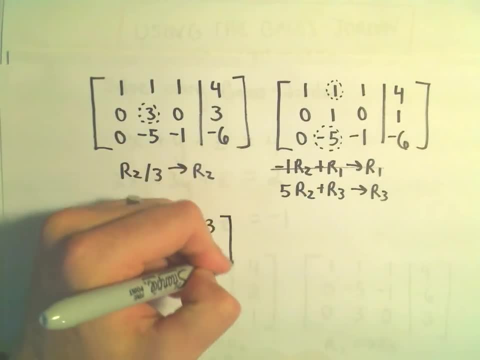 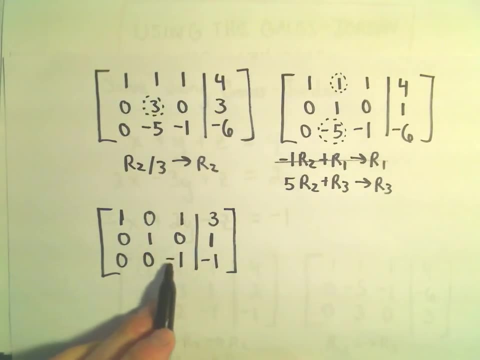 5 plus negative 6 is going to be negative 1.. Okay, so the next thing we would want to do is we want to make our negative 1 into a positive 1, but we could just take negative 3, or negative 3,. 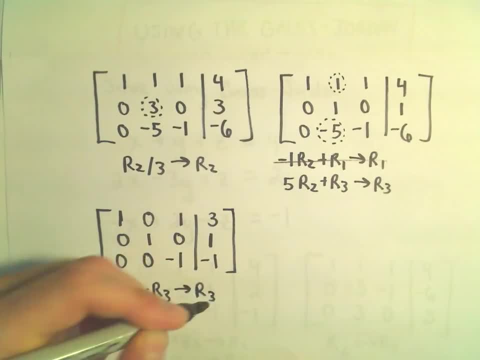 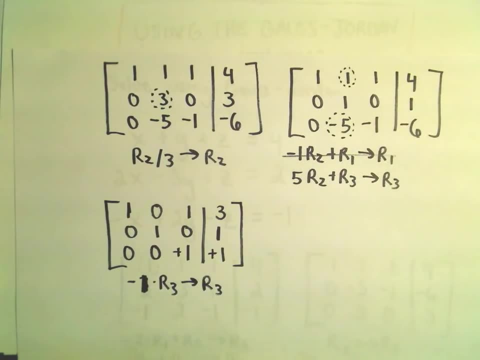 negative 1 times row 3 to get our new row 3.. And I'm not going to rewrite all this. All that's going to do is make those into positive 1s, I think the last thing I'm going to do now. okay, so we want to make our positive 1 into a 0.. 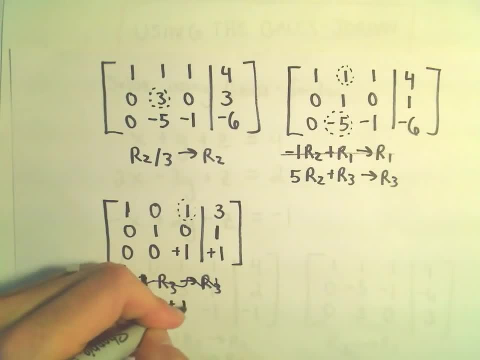 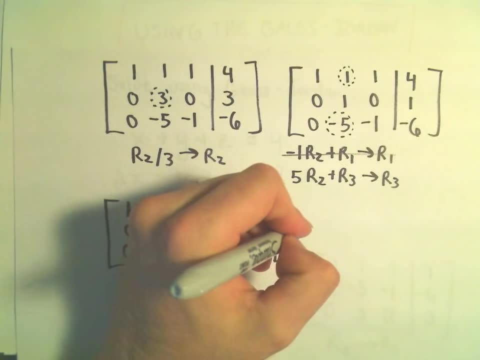 So I'm going to take negative 1 times row 3, add that to row 1 to get my new row 1, and then I think we'll have our solution. So let's see, the second row is staying just like it was. 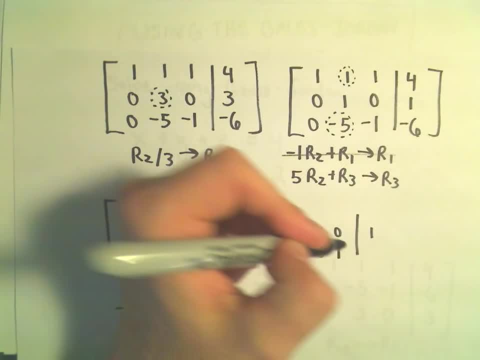 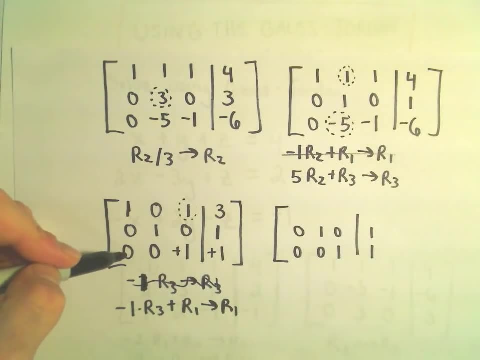 The third row is also staying just like it was, And if I take negative 1 times row 3 and add it to row 1, we'll get negative 1 times 0, which is 0, plus 1 will be 1.. 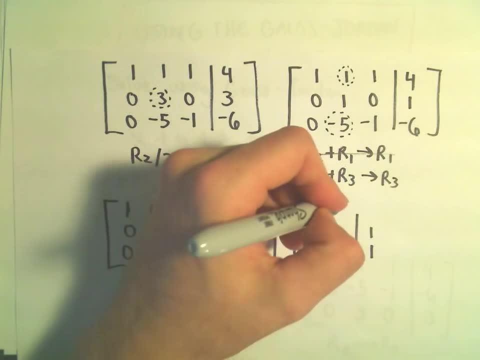 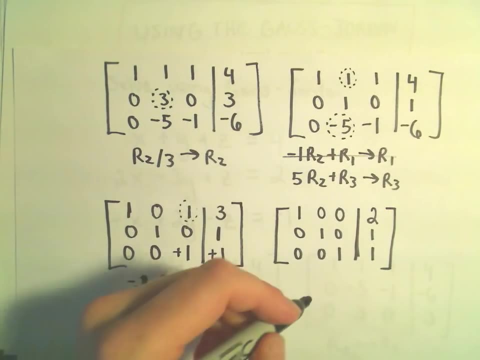 We'll get 0 plus 0,, which is 0.. We'll get negative 1 plus 1,, which is 0.. We'll get negative 1 plus 3,, which is positive 2.. And now we've got our solution. 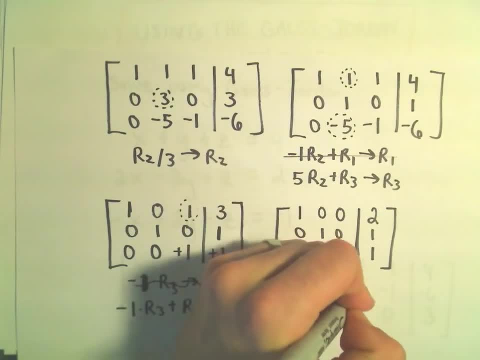 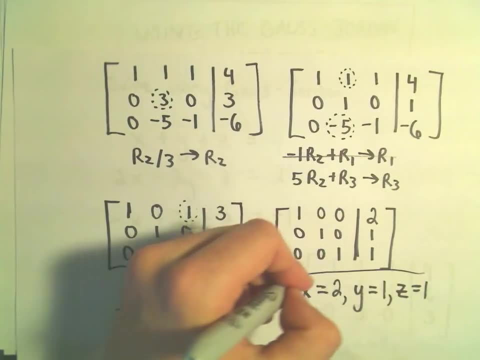 It says: 1x equals 2., 1y equals 1. And 1z also equals 1.. So again, you can always go back and check if you plug in 2 for x, 1 for y and 1 for z.